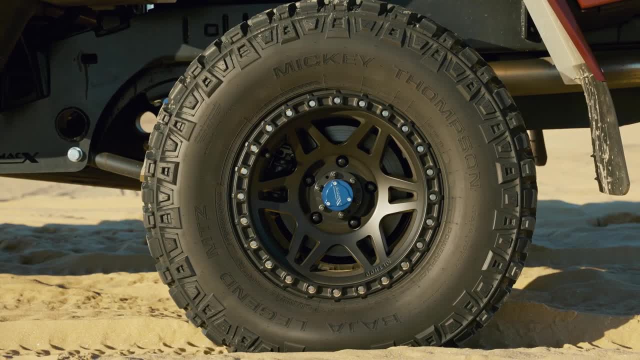 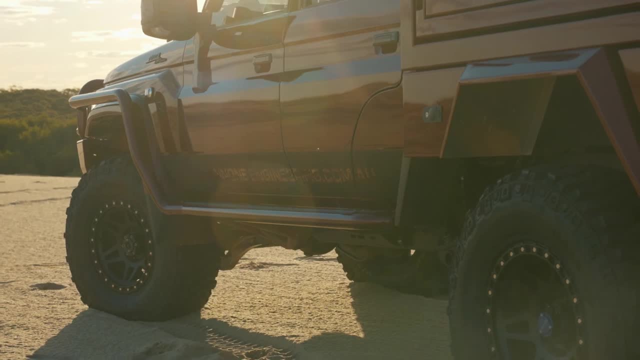 and went with the Method 312s. As far as the color combination, I've gone with straight black. I'm trying to introduce as much black into the accessories and wheels as I can. And then the Method 312s. they're wrapped in the Baja Legend. 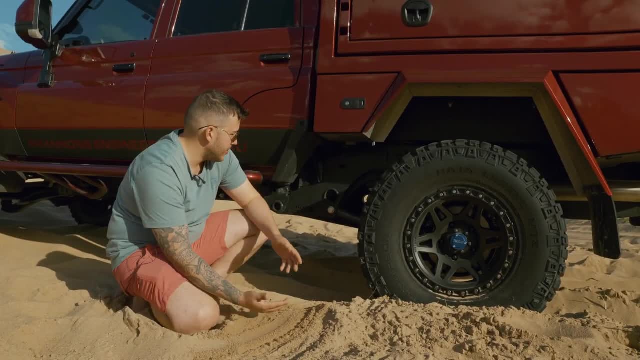 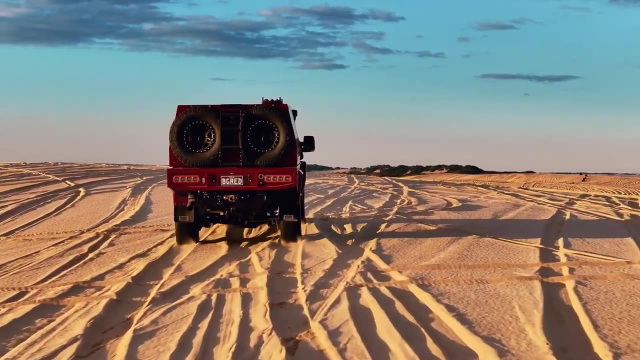 MTZs from Mickey Thompson. So, moving back to the suspension and the GVM upgrade, we're running a full coil-converted rear. Today we've just been driving up and down the dunes and it's just been so comfortable. So we're running J-Maxx's. 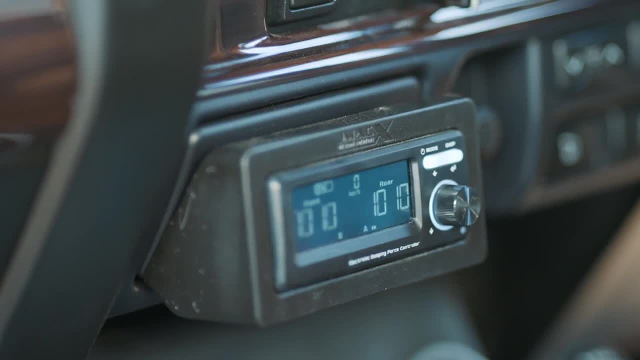 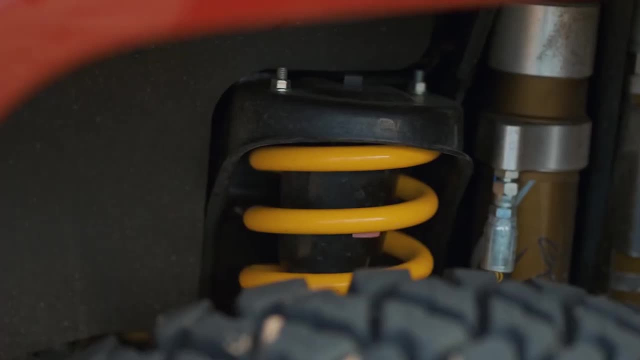 new Alpha electronically adjustable shocks Going on the beach. obviously we can just quickly soften them and then get back on the beach. Once we're back on the tarmac we just stiffen them up. So part of the J-Maxx. 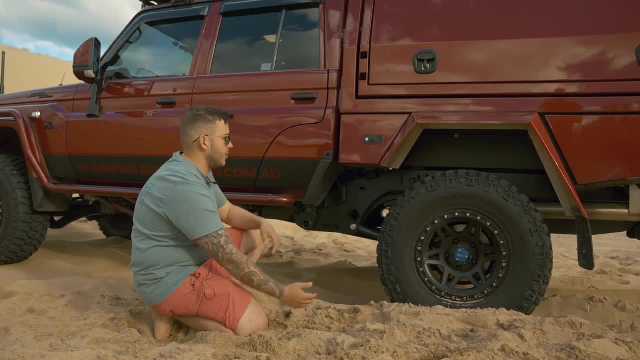 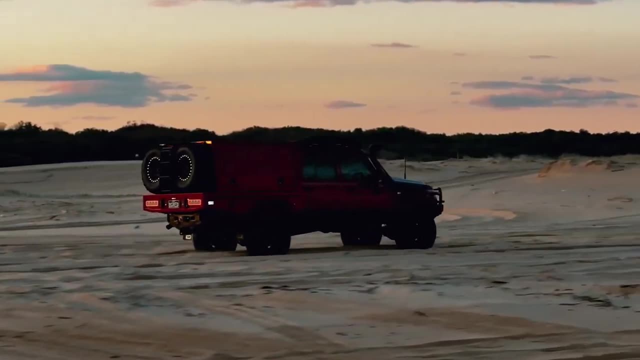 4495 GVM upgrade, you get a 300 mil extended, completely new chassis which actually brings the wheelbase back 300 mil as well. So our axles are centered with our canopy When we're driving on the beaches or wherever this will be. 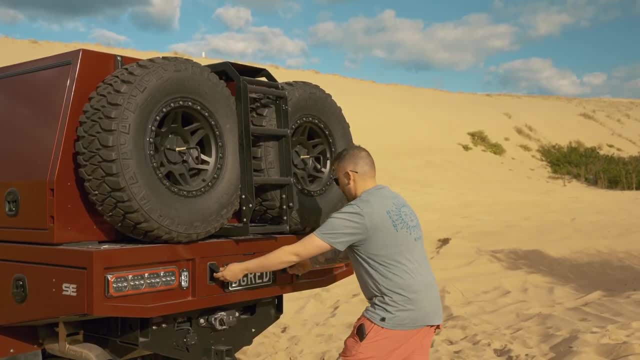 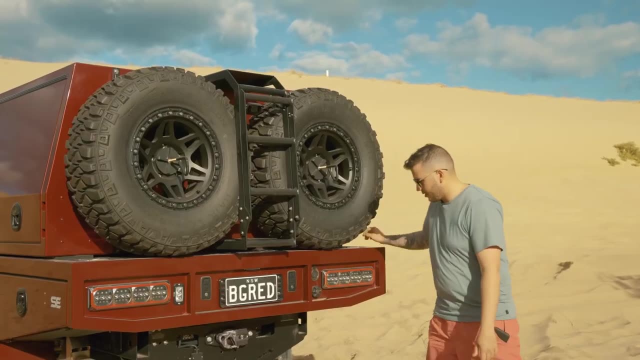 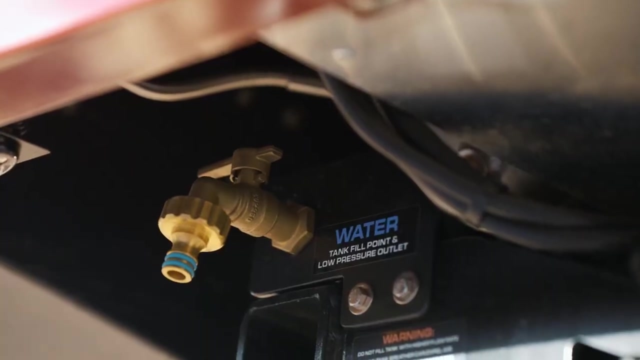 able to handle it a lot better off-road. Future plans for this will be to introduce an induction cooktop here. So at the back here the chassis, we have a gravity feed here as well as a diesel. We also have a water outlet here, And underneath here we have a water pump. 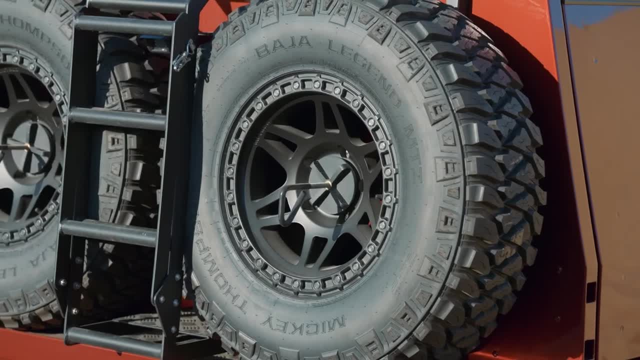 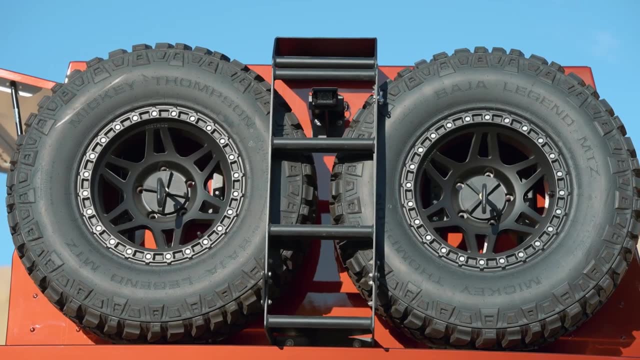 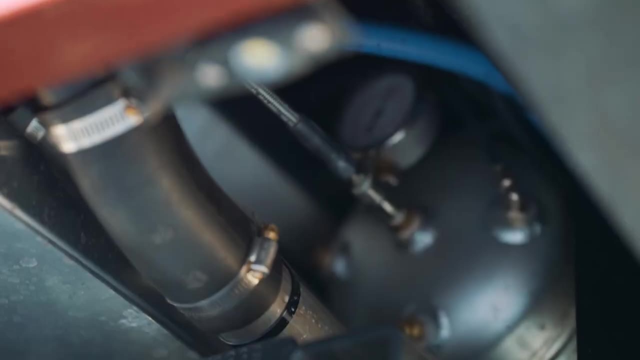 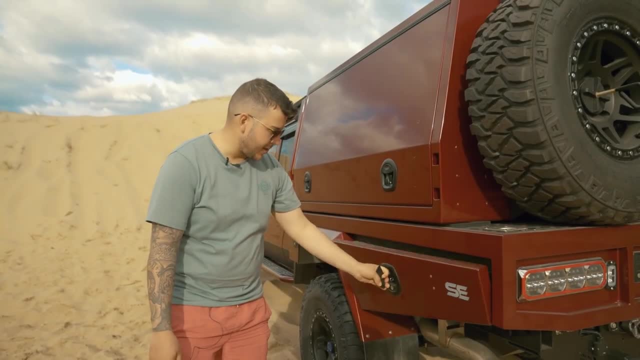 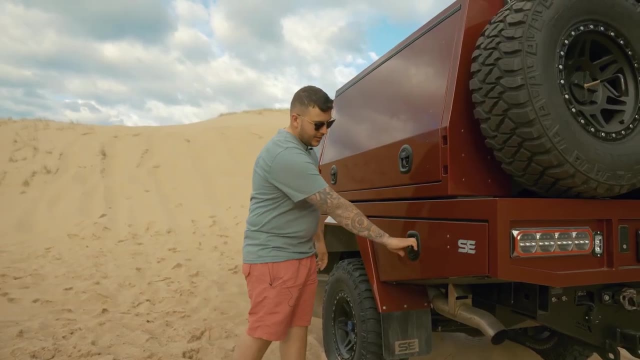 it's just a very quick process. So, moving back here, we've got four compartments, We've got two smaller toolboxes and then two bigger ones in the back. This side we are using an ARB twin compressor And then I've got all my 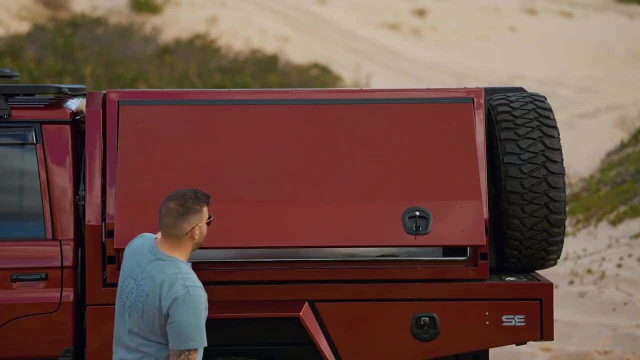 air hoses in there, Colour-coded canopy from Shannon's Engineering which is full aluminium. I have no idea what I want to do in the back here. There's so many options. I'm just going to keep it blank for a little bit and make up my. 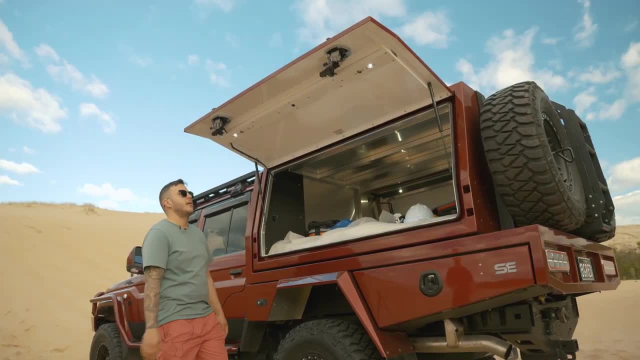 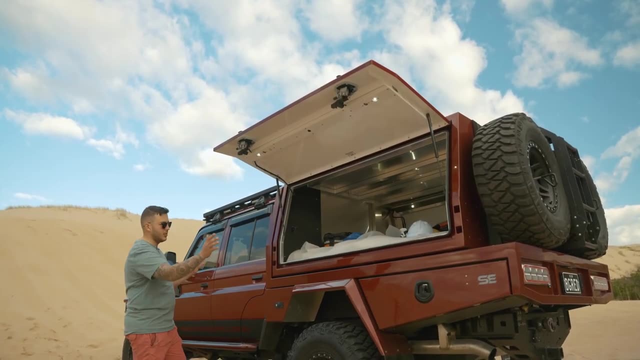 mind eventually. So on our doors we have motion-sensitive lighting And then, if you want, you can choose amber lighting. We have these points either side where we can lift the canopy off and use the full 2.1 metre tray for its uses. The whole car is covered in PPF wrap That 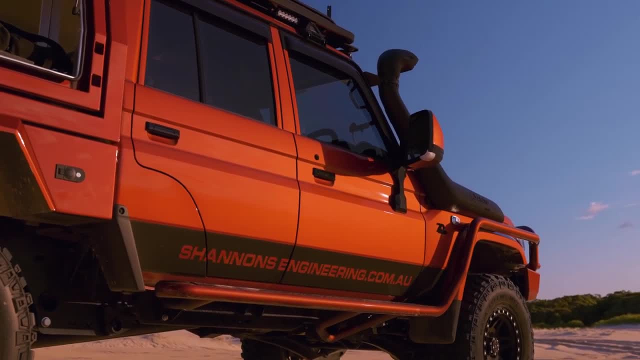 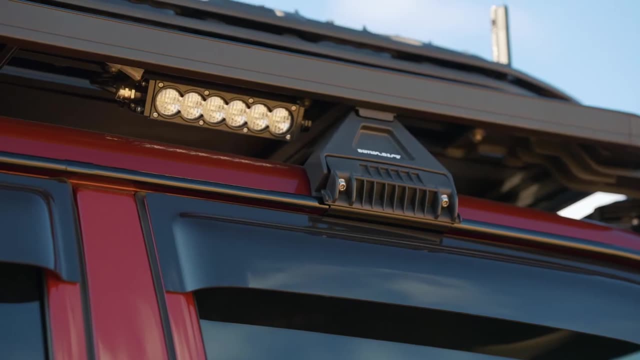 was done by Australian Detailing Services. Hit up Ryan if you ever want your car to look as good as this. Ryan from Oz Detailing. he also painted my door handles and my gutters. Big thanks to him. I have chosen the Clearview. 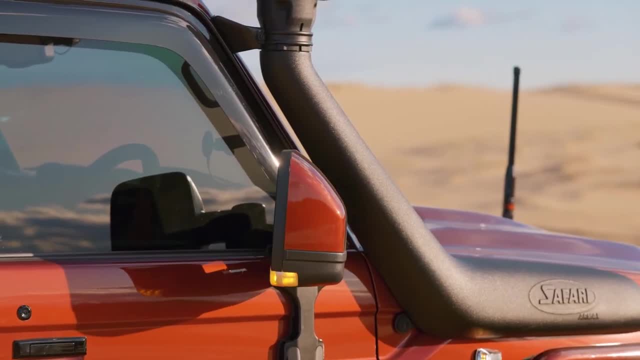 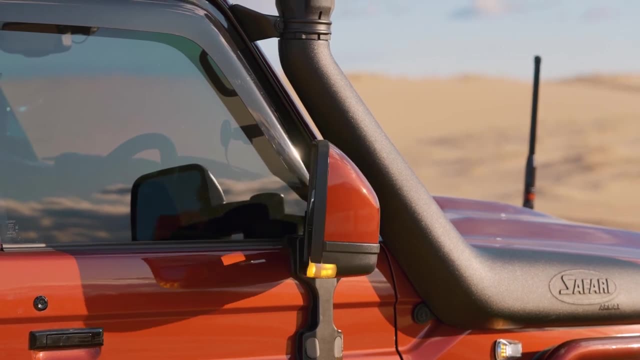 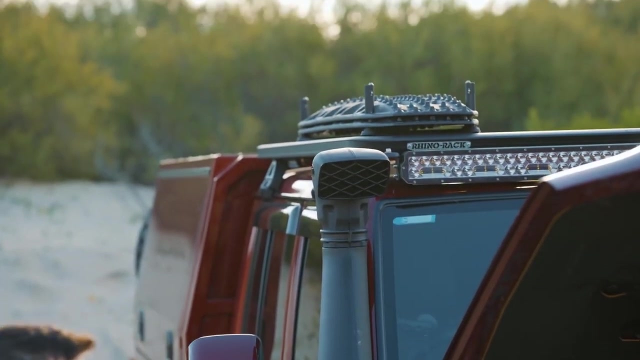 Next Gens with Powerfold and the indicators. So awesome when going into the scrub. So much easier than having to pull your mirrors in and just quickly Powerfold them in, and then you're done. So here at the front we're running a Safari Armax snorkel along with a GSL air box and GSL intake pipe. 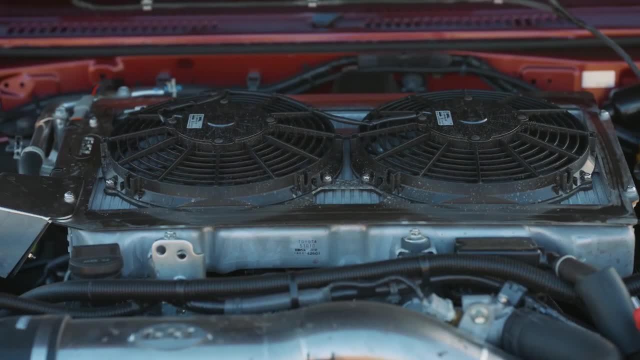 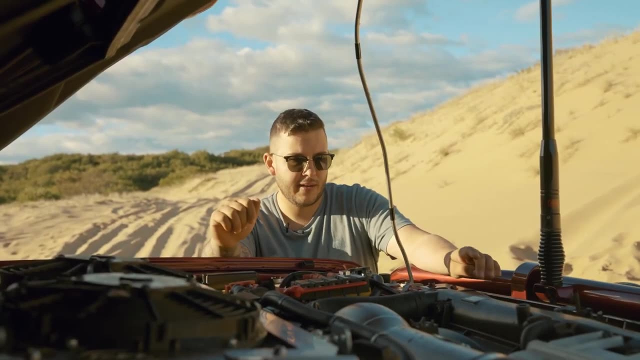 And we're also running their fan kit. just to keep it cooler, We've got a dual battery setup. This is mainly controlling the cab and the tray, And then we've gone with Redarc, their BCDC charger, to look after that. We're running. 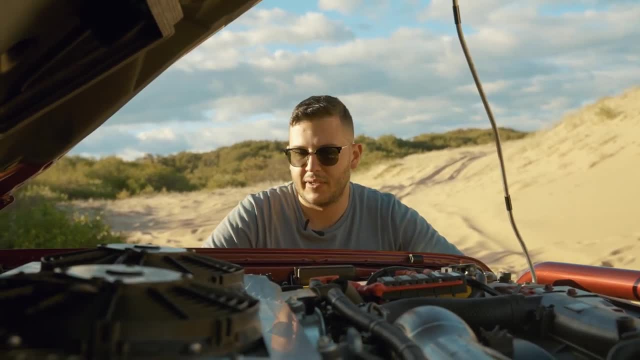 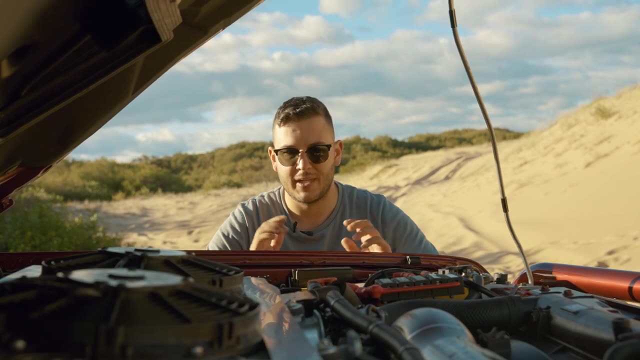 just the basic tune on the engine, We're making 550 Newton metres of torque at the wheels, which is awesome on 35s, especially with the extension. Future plans for the car will be to run a G350 turbo and see if we can get up to a. 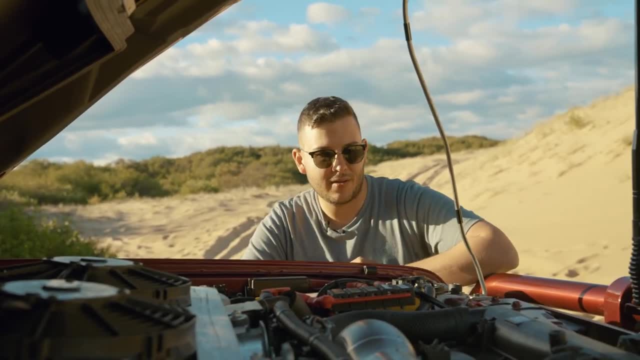 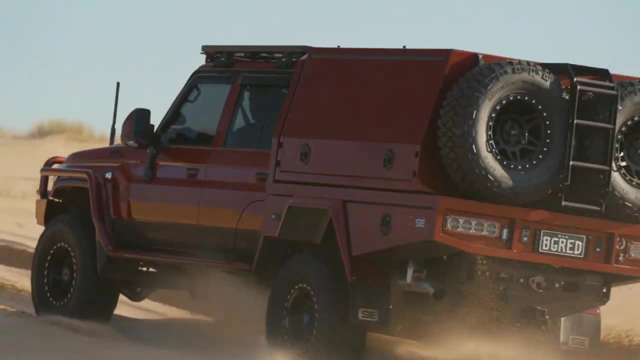 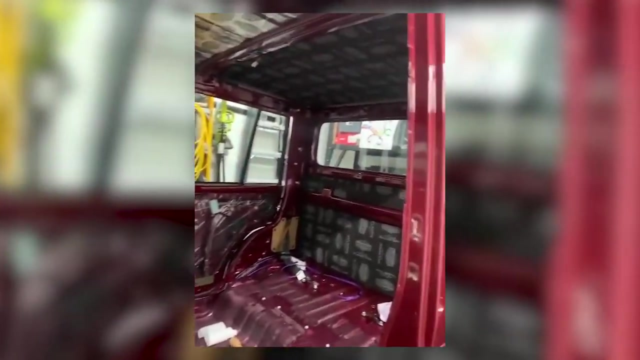 thousand Newton metres of torque just so I can rip up Stockton Beach better. So in the interior the whole cab has been soundproofed. Centre console from Department of Interior, Future temperature gauges to go in With the 70th. 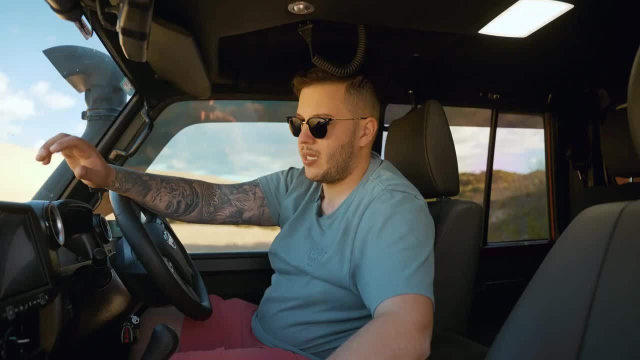 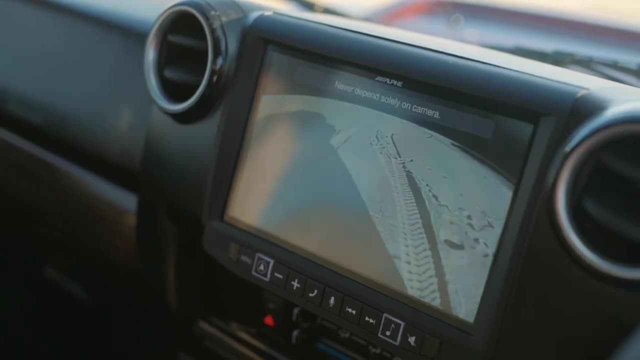 anniversary. you get this nice wood grain finish, And instead of keeping the original head unit, I've put an Alpine X903D in here, which is a really good bit of kit. That canopy camera on the back is hooked up to our monitor here, So 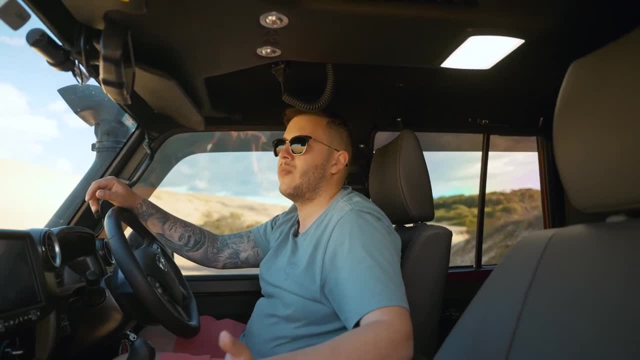 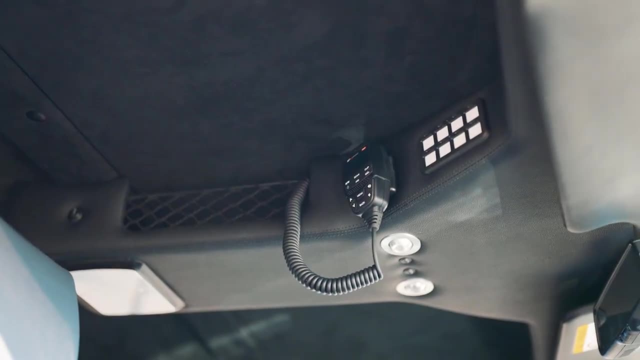 when I'm driving, I can always see what's behind me, or if I'm reversing, where there's trees Or anything like that, that's all showing up in here. This is another piece from Department of Interior which is awesome. Heaps of storage here And then.